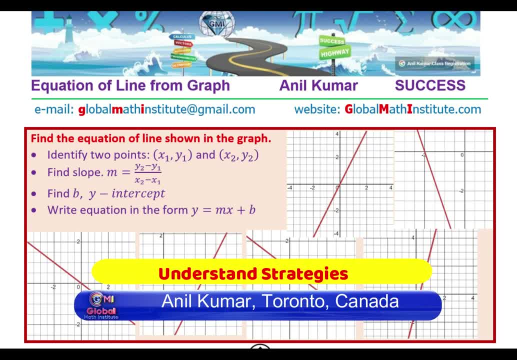 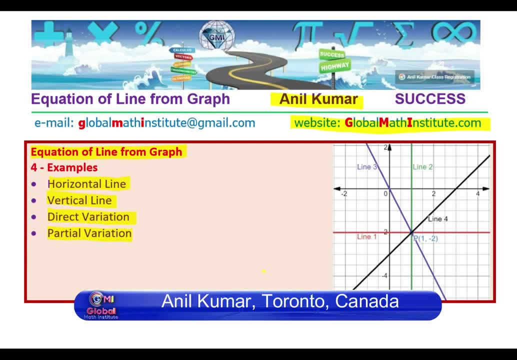 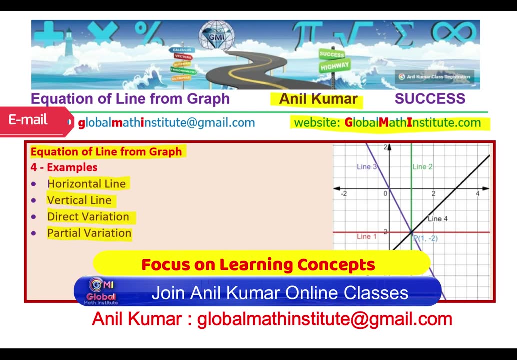 For example, this one right. So we had six examples in that case And we wrote the equation in the form of y equals to mx plus b. Now, in this particular case, we are going to understand a few things more, And you will also get to know how do we immediately write down the equation of the given line. 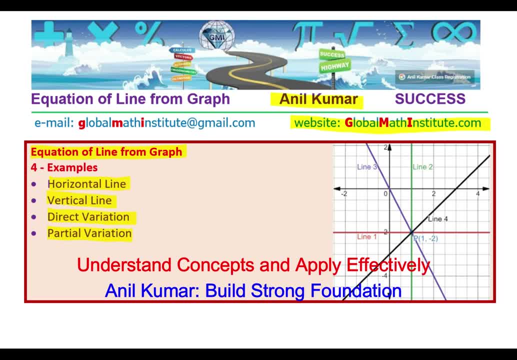 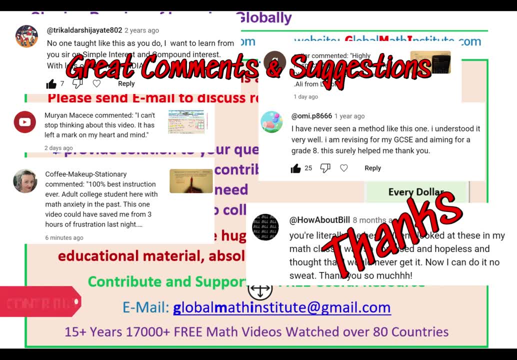 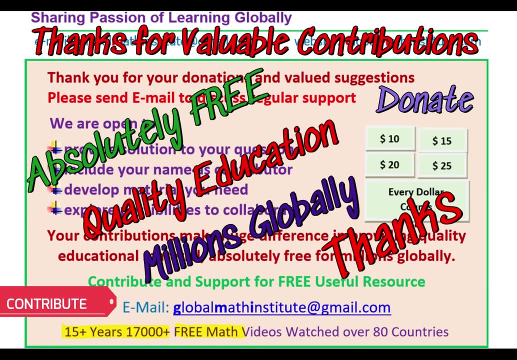 So some shortcut methods, right, Okay, great. Let me also thank all the viewers and subscribers for watching the videos, posting excellent comments. You know, since last 15 years we are providing you with absolutely free services. We have 17,000 plus videos so far which are being watched over 80 countries. 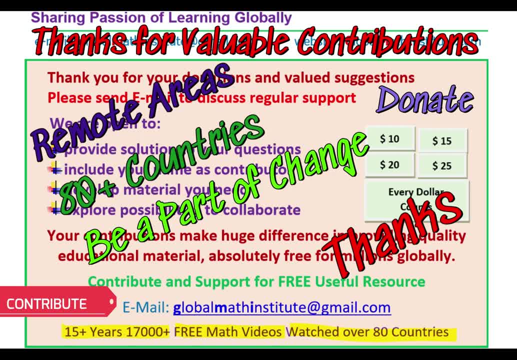 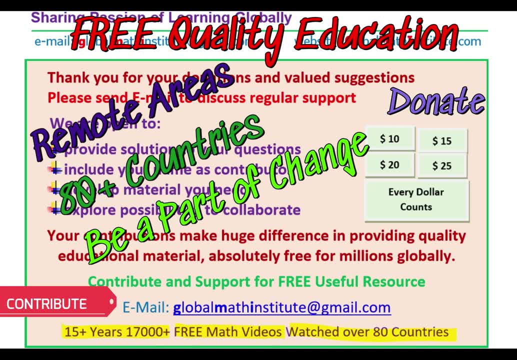 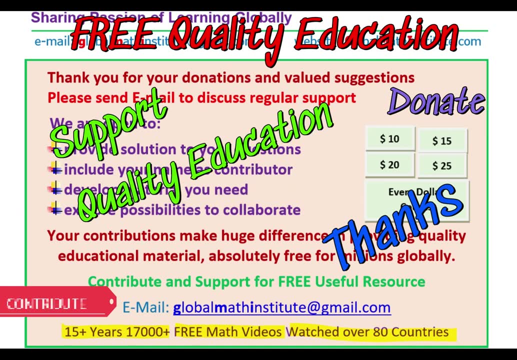 Quality education for all, Absolutely free. quality education for all. Quality education for all is our motive And we need your support for that correct. So thanks for your support. Anytime you're ready, you can support. Every dollar counts Great. 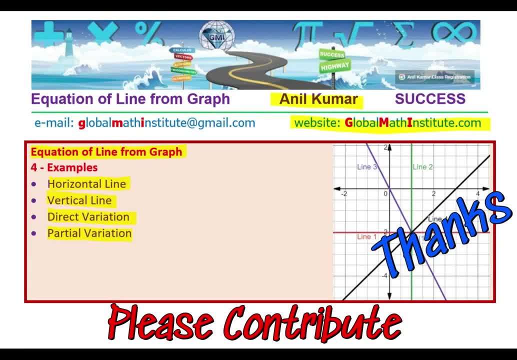 So let's get back to our topic: Current video, in which we are going to write down equations of four given lines. you see line one, which is a horizontal line, and then line two, which is a vertical line, and then we have a line three, which is that variation, and line four, which is a partial variation. 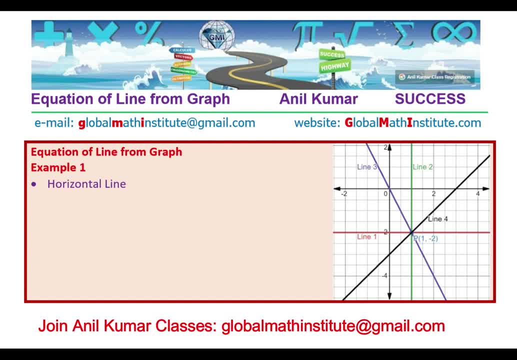 So question number one: how do we write the equation of a horizontal line? So generally we write the equation in the form: y equals to mx plus b. Now if the horizontal line is being considered, which is right there, you will notice that it goes through a point p which is 1 minus 2.. 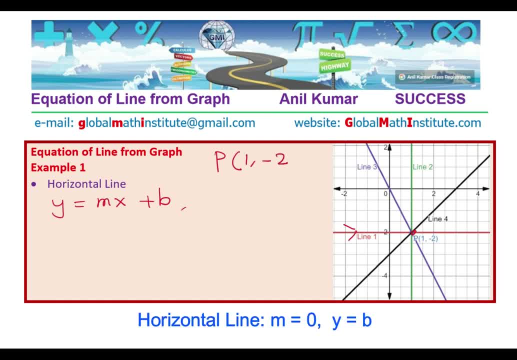 So it is going through a point p, which is 1 minus 2.. So you see that at every point the y value is exactly same, Y value is exactly same and y is equal to minus 2.. So that becomes the equation of the line. 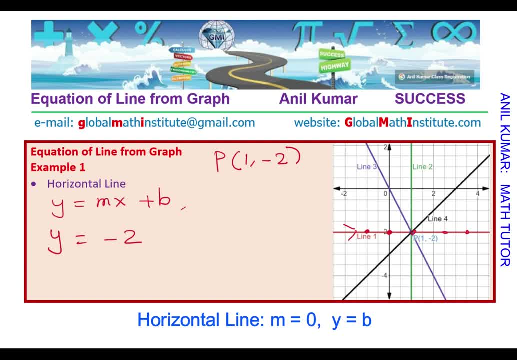 You see, the y intercept is also minus 2, right, And what is the slope here? Well, slope is 0, since it is not at all rising Rise over run is slope right. So consider m as rise over run. 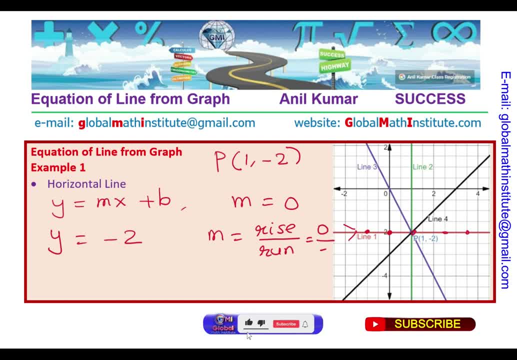 Now, since rise is 0, so anything here will make it 0, right? So that is one reason m is 0. So we are looking only for the y intercept, y intercept being minus 2, and everywhere along this line, as you can see, y value remains constant. 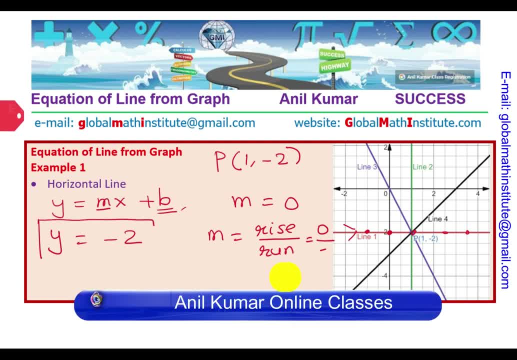 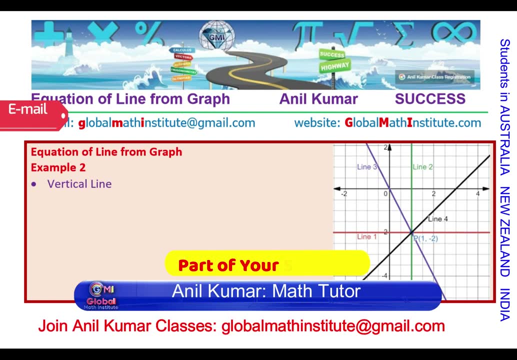 So it is the constant value of y which gives the equation of a horizontal line. So, in general, horizontal line will be the y value of the line, correct? Well, let's extend the same concept to a vertical line. Vertical line, in this particular case, is line 2.. 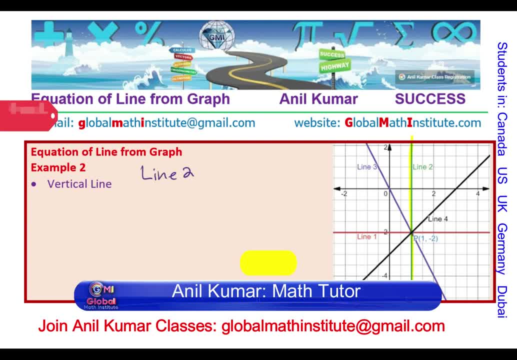 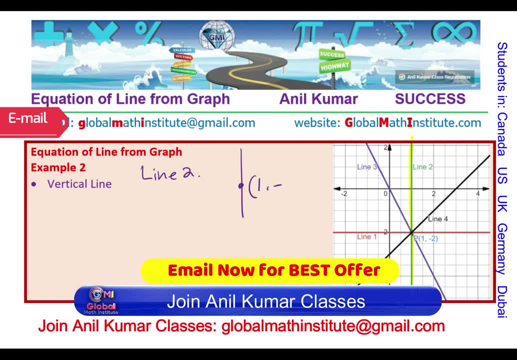 So, as you can see, line 2 is a vertical line which passes through a point which is, in this particular case, p 1 minus 2.. So you see, at every point, x value is what It is: 1.. 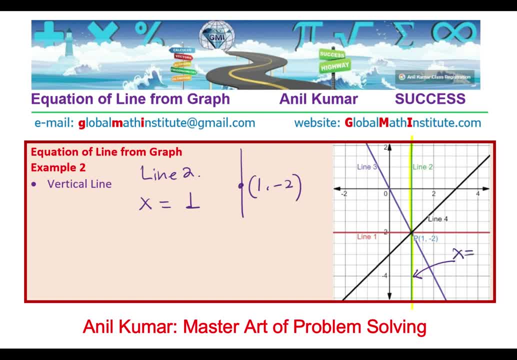 And therefore the equation of this vertical line is: x equals to 1. Makes sense. Now, an important thing to understand here is that you cannot really write down the equation in the type y equals to mx plus p, since what is the slope here? 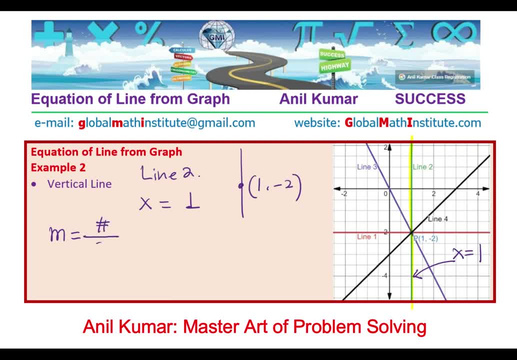 Slope is something right over 0.. Now, this is undefined, right? Do you see that, Since the slope is undefined, we cannot write equation in the form y equals to mx plus p? The only equation which you can write is the x value remaining constant, right? 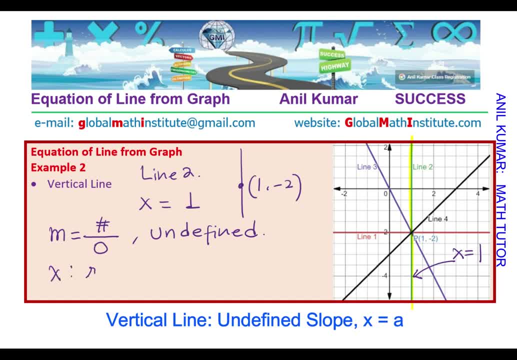 So, as you can see here, x remains constant, right, And that gives you the equation, which is: x equals to 1, in this particular case, when the line is passing through the point p, which is 1 minus 2.. 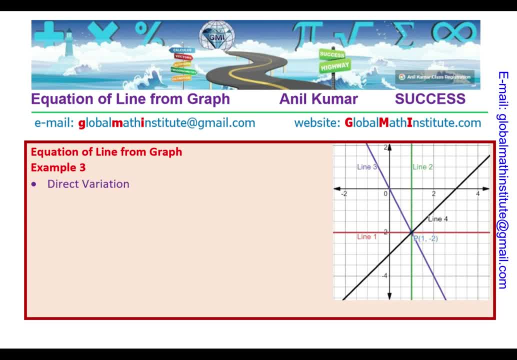 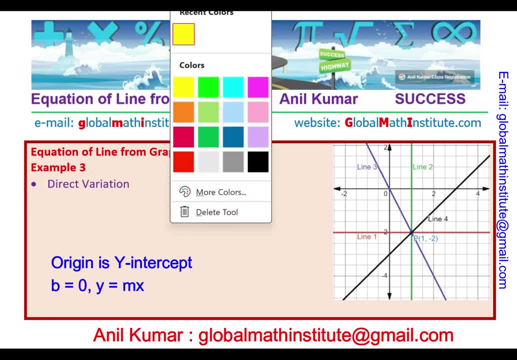 Makes sense, right? Well, the next example- question number 3, is a direct variation. Direct variation really means that the line passes through origin, right? Do you see this line, which is Line number 3. It passes through origin. 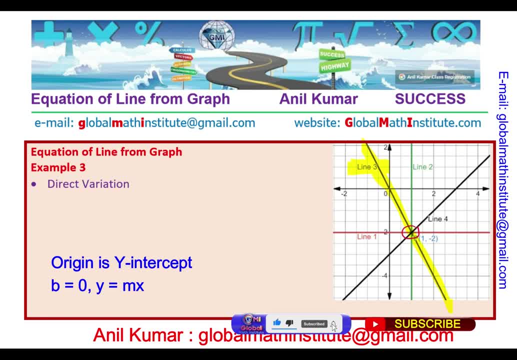 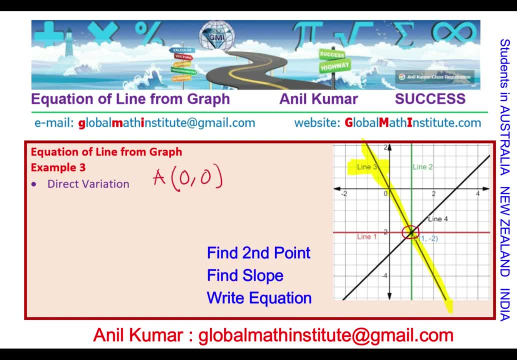 And more than that, it also passes through a point p which is 1 minus 2.. So there are two points on it, One a, which is 0, 0, very well defined, And then we have a point p, which is 1 minus 2.. 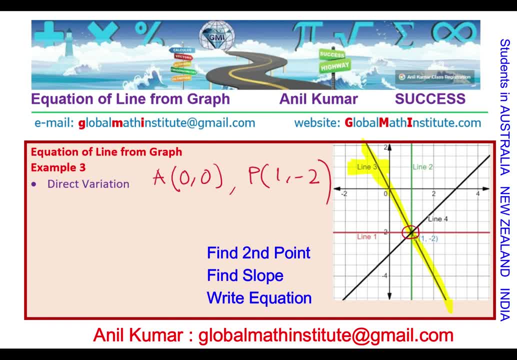 Now, using these two points, we can always find the slope. So what is the slope here? Slope in this case is y2 minus y1 over x2.. Y2 minus x1, which is minus 2 minus 0, over 1 minus 0, which is minus 2, clear. 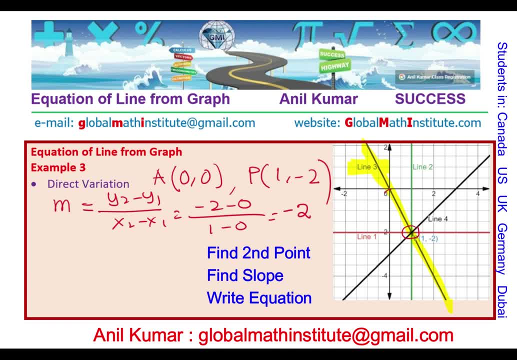 The line going down right. You can always see it goes two units right, 1,, 2, and then one unit towards the right. So the slope is minus 2.. Since the y-intercept is the origin itself, the equation of the line is: y equals to m times x, right. 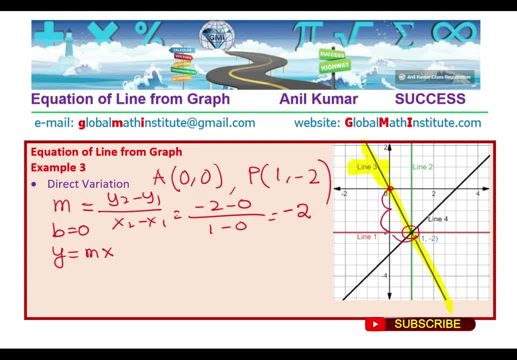 Since we know b equals to 0, right, So we can write down this equation As y equals to the slope of minus 2 times x. correct, So directly we can get the equation, Since we know the y-intercept, right? 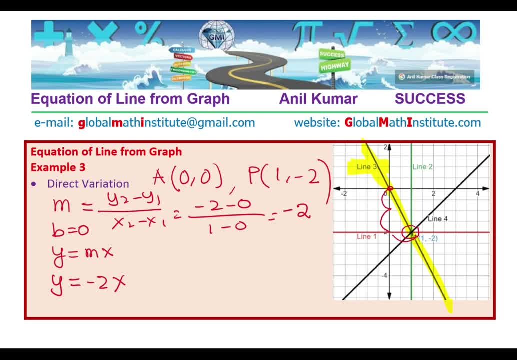 And the slope. we just calculate it as minus 2.. It's a direct variation as it goes through the origin. So I hope till now everything is absolutely clear. You may, if you want to learn from me directly, send an email on globalmathinstitute at gmailcom. 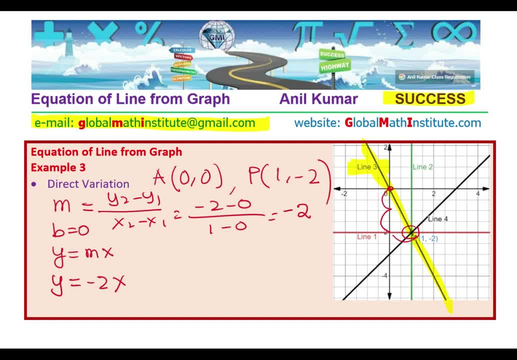 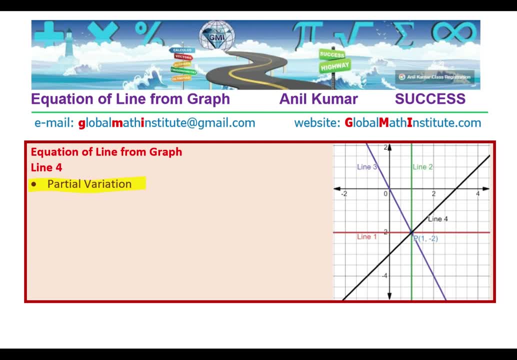 Our students will be able to learn from you. The students are right there on the top doing extremely well. You can be there. Well, here is the last question. We're talking about partial variation. Partial variation means that the line is not going through the origin. 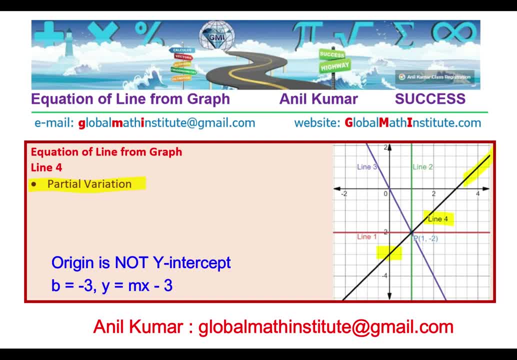 Do you see this line, which is line number 4 for us? It is passing through a point on the y-axis at minus 3.. So here the value of b is equal to minus 3.. That is the y-intercept, right. 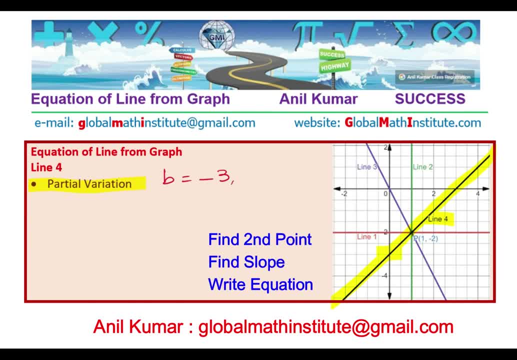 In this case, the y-intercept is minus b, right? So the equation y equals to mx plus b can be written as mx minus 3.. We need to find the value of m. Let's consider two points. So one is the y-intercept, which let me call this as a and which is given to us as 0 minus 3.. 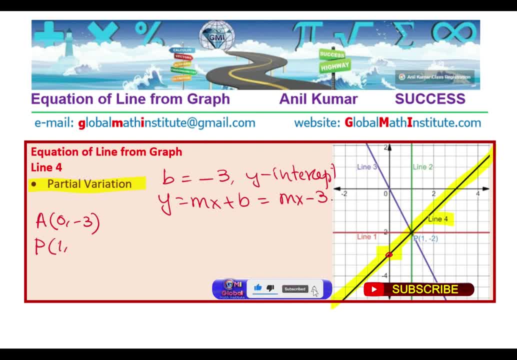 And the other point is 0. And the other point p, which is 1 minus 2.. Now from here you can find the slope m, which is y2 minus y1 over x2 minus x1. And clearly it is minus 3, minus of minus 2, over 0 minus 1, which is minus 3 plus 2 over minus 1.. 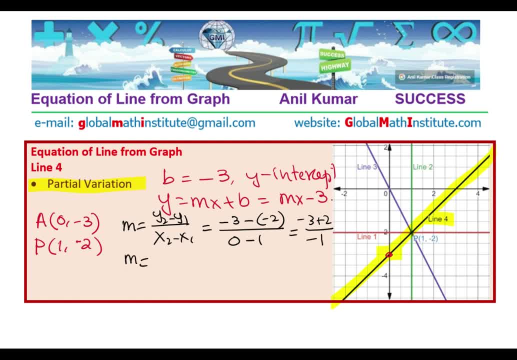 And that gives you a slope of Minus 1 over minus 1, which is plus 1.. So you can see the line is rising. It has to have a positive slope, being 1 in this particular case, And we know the value of b is minus 3.. 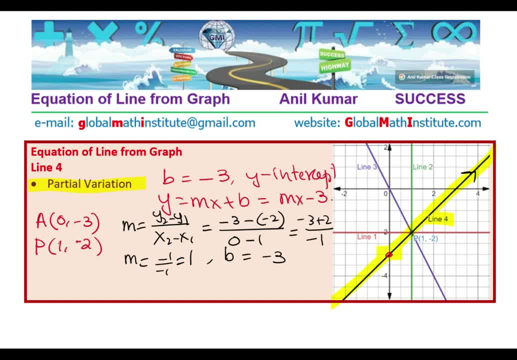 And therefore the equation is what? Well, clearly, the equation will be: y equals to 1x, right? So we don't write 1 here, x minus 3.. That becomes the equation, Do you see that? So in this particular case, we have seen four special examples. 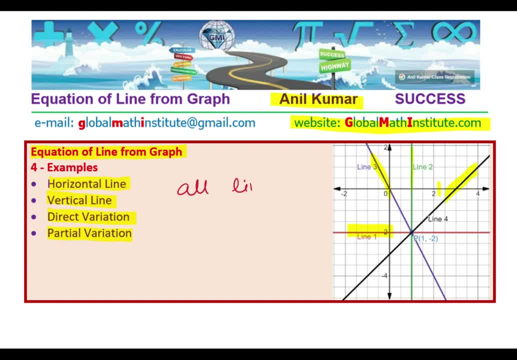 All lines are going through, which point? Through point p, right, And point p is 1 minus 2.. So horizontal line, if I see, is 1, in which y value is constant, correct, And vertical line, x value is constant. 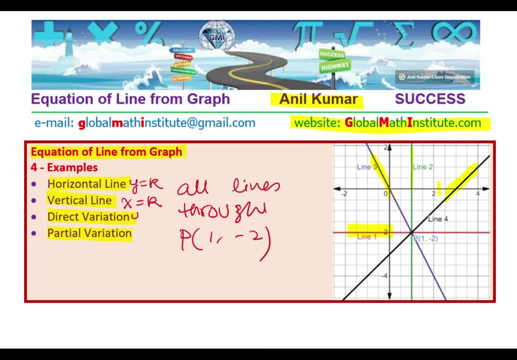 That is kind of important to understand. In direct variation we have y equals to some constant times, x, where constant is the slope, And a partial variation is a general line which is written in the form: y equals to mx plus p, where we need to find the slope right.